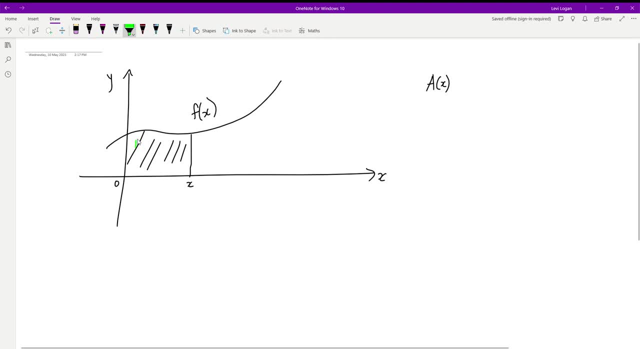 into this function here. it will give you this area here. So this green bit here, Okay, And now let's consider a bit. So if we were to extend this okay to some distance, let's say a really small distance, h So up to, let's say, here, where this would be, this distance here, along, here is. 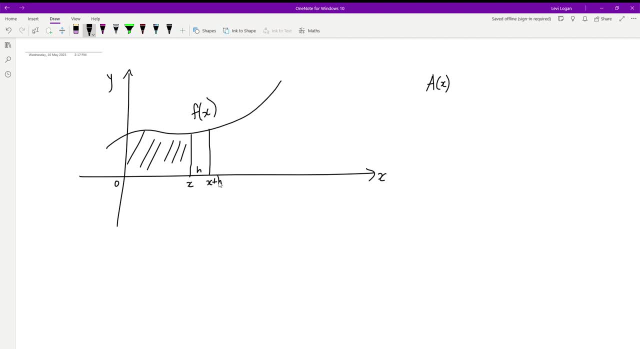 h, And this would be h plus x plus h. Okay, So then the area. up until this point here. so this whole blue bit would be the area, but you input instead of x. you put an x plus h, don't you? So if you input this point into this function here, it will give you that blue area. 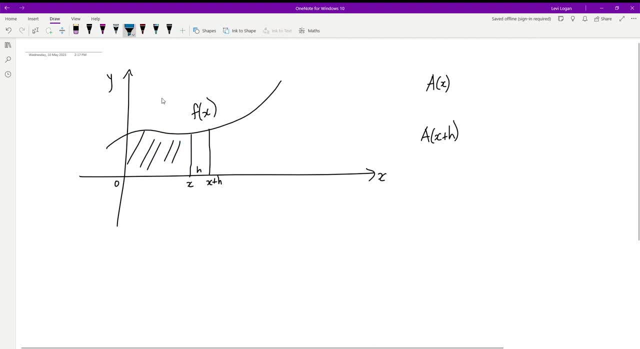 Okay, Now, let's say we wanted to work out an expression for just this strip here. Okay, So just this light blue strip here. Well, that will be this area, So this whole big area. subtract this little area here, wouldn't it? So it would be a of x plus h minus a of x, Okay, 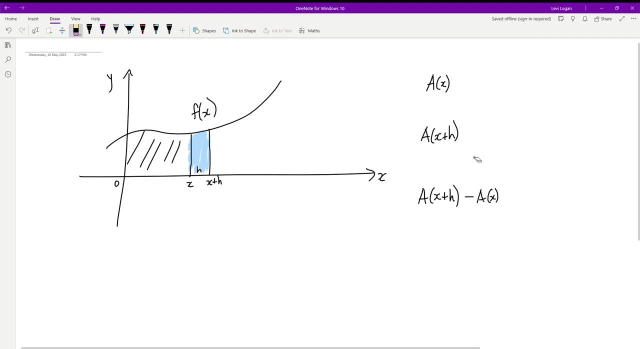 So that's our blue little area. Now let's take a look at it here. Okay, So let's just say we're zooming in on this rectangle here, So it looks something like this, doesn't it? That's a terrible drawing. I'm just going to scroll down real quick. 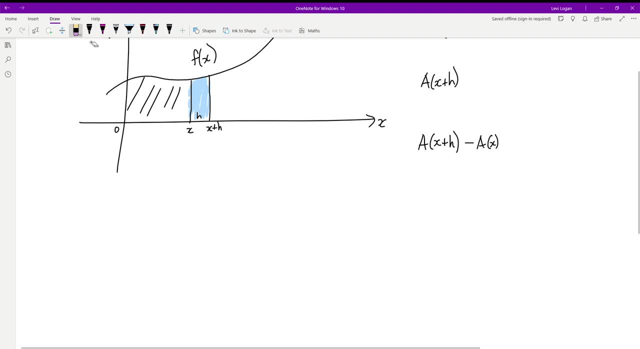 And let's make a better representation of it. Okay, So this is our little strip here. So this is our blue strip. Okay, Now, this distance here on this rectangle is h, But let's consider this little bit at the top here. Let's say we only wanted the rectangle up until this height. 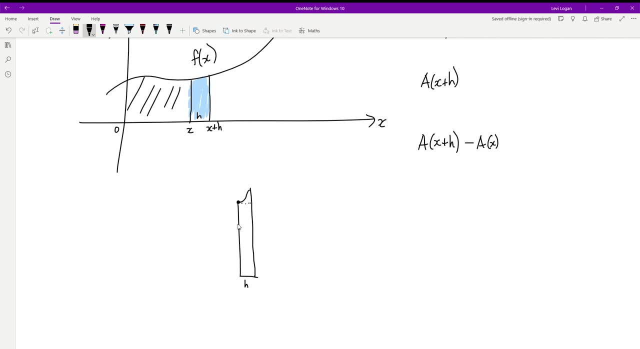 here. Okay, What would this height be? Well, if this curve is f of x, the height at x is going to be f of x, isn't it? So it would be just normal f of x because an input and this is your output, pretty much. So this is: y equals f of x. 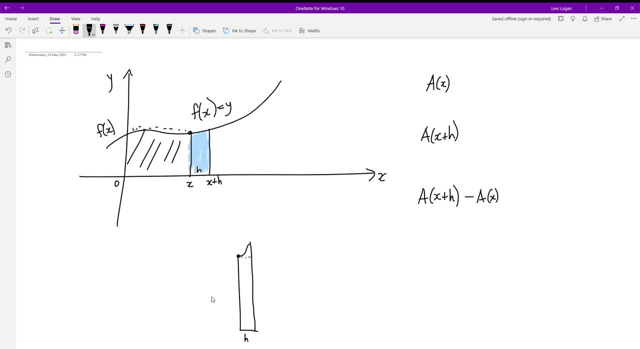 So this height here would be f of x, wouldn't it? Okay, So now this is the area we're looking at here. So this green area, just in up until this height here. So we're we're ignoring this little bit here. this area here will be f of x multiplied by h, wouldn't it? 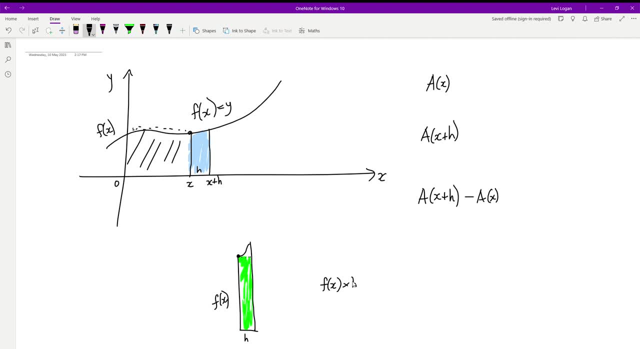 okay, now this area here is going to be less than this blue strip, isn't it? so this is our expression for our blue strip. so f of x multiplied by h is going to be less than or equal to our blue strip here, because this bit is our blue strip, but this is a little bit here. we're not. 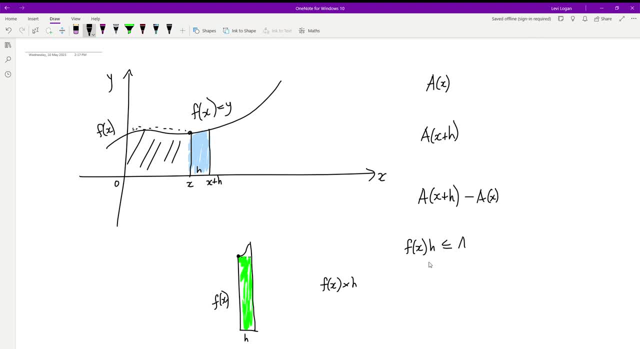 counting for. okay now, so this can be less than this expression here. okay, so far, so good. and now let's take the bit. now. let's say we wanted to work out- not pretty much- this bit. we wanted to look at this height here as well, so the height up into here. so this bit here would be what would. 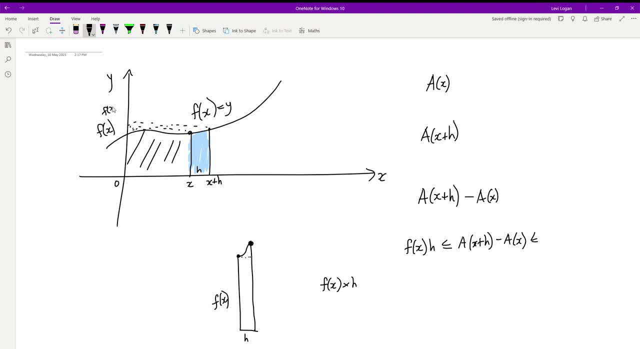 that be? that would be f of x plus h, wouldn't it? so this would be f of x plus h. now, this would give us the area of this. so we're getting a bit more than our blue rectangle, aren't we? so what we can say here? 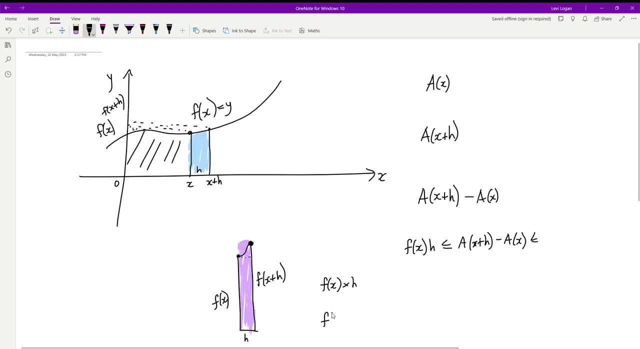 is that the area of this purple bit will be f of x plus h multiplied by h. now, this area here is going to be bigger than our blue bit, so we can say that this here is less than or equal to f of x plus h multiplied by h. now, that was the hard bit, getting this expression here. so now i'm just 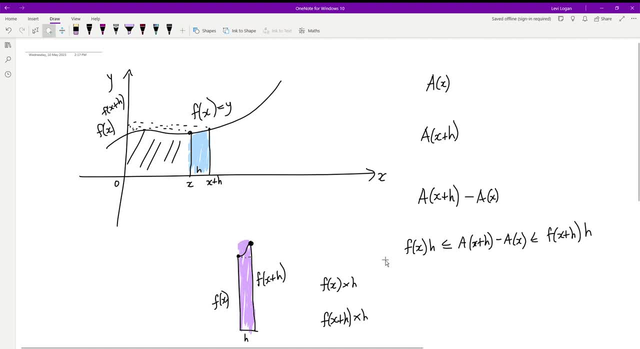 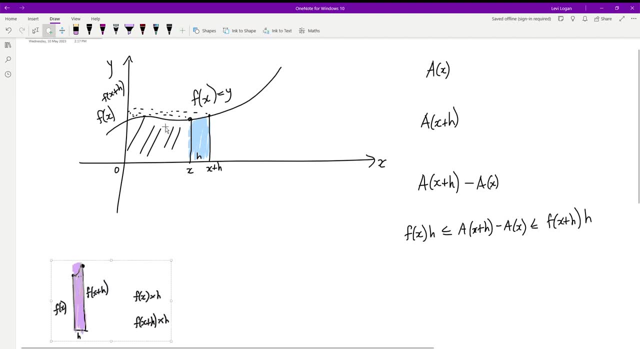 going to remove. well, not remove this, i'm just going to move this stuff to the side here because it's not that important anymore. getting this set up was more important because we have a graph here. okay, now we can see we have h here. we have h here, so we can divide. we have basically, you have a. 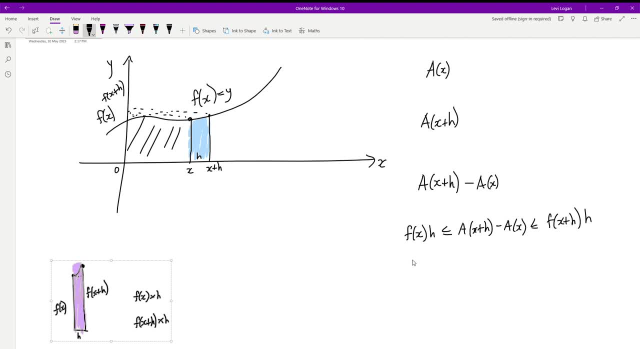 triple inequality here. so if we divide by h on all three, then we have a triple inequality here. so we're going to have f of x, a of x plus h minus a of x over h to your f of x plus h. now what we're going to do. 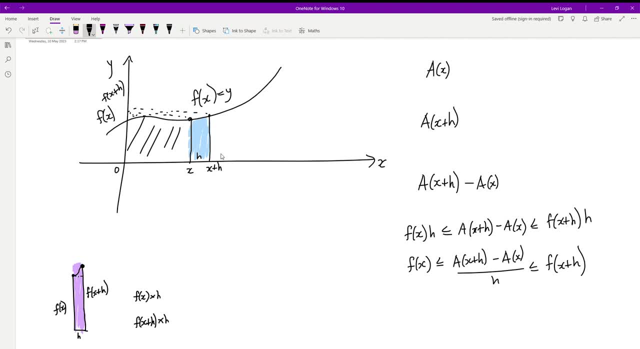 is basically, we're going to apply a limit, we want to basically make h, we want this distance to be as small as possible. okay, now the reason we want to do this? because if we do this then we'll have basically, um, a dash of x in our expression. so if we apply the limit, 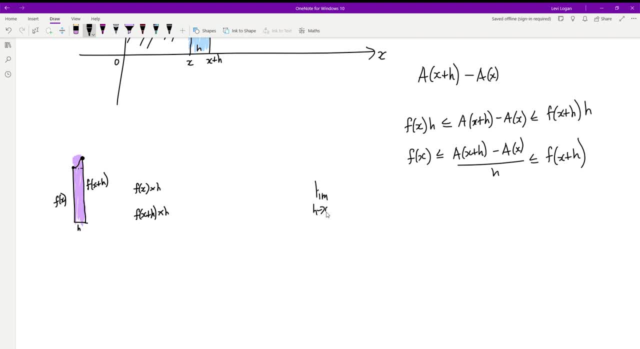 as h goes to zero if we apply to this side. this side isn't going to change at all, so that's still going to be f of x. if we apply it here, we're going to have the limit, as h goes to zero, of this expression here. now i don't know if you recognize this, but this is actually the first. 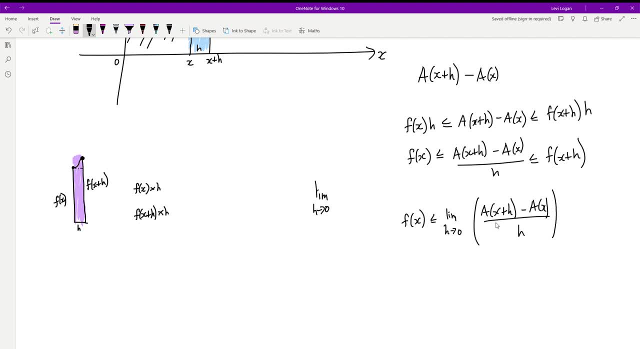 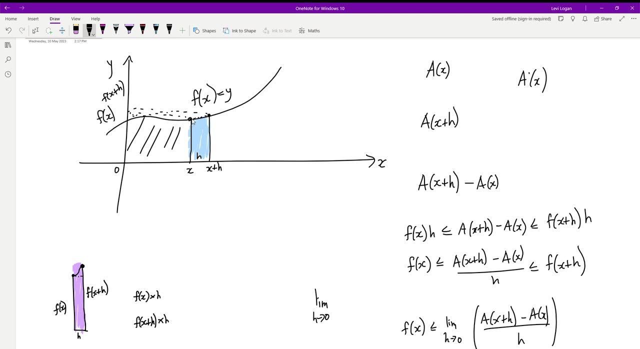 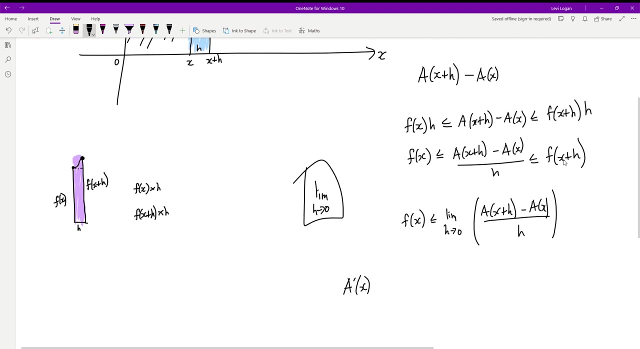 set ofamous principles. so in other words, what we have written here is a dash of x and here this bit here. so f of x plus h. this bit is a bit funky. so as h goes to zero, this point here is going to travel along to become f of x, isn't it? so if we apply this limit to this bit here, that's just. 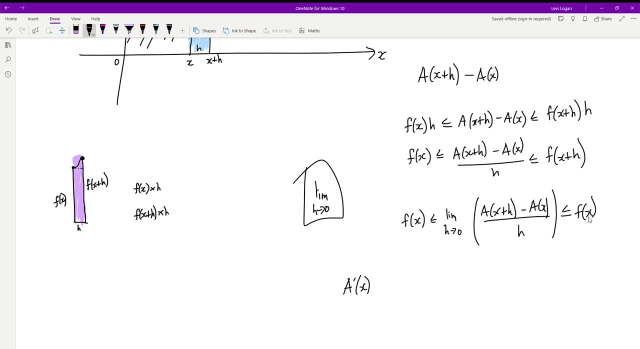 going to be f of x. and now we know this bit is a dash of x, and that's normal. if we demon ELM, it's only puh. even smalllles spread f, a dash of x, so we can replace this as f of x. oh whoops. f of x is less than or. 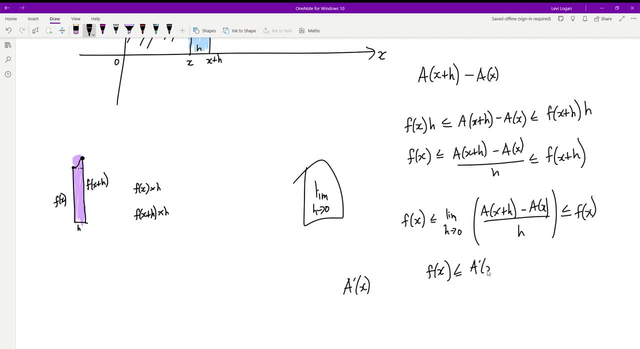 equal to a dash of x. So a dash basically means it might be written another way. is the derivative with respect to x of a okay is also less than or equal to f of x. Now, if something is less than or equal to f of x and something is also greater than or equal, 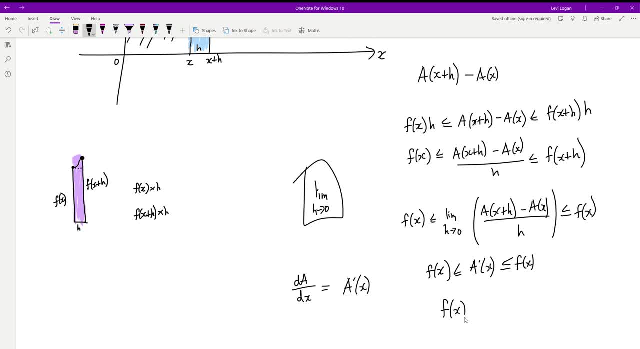 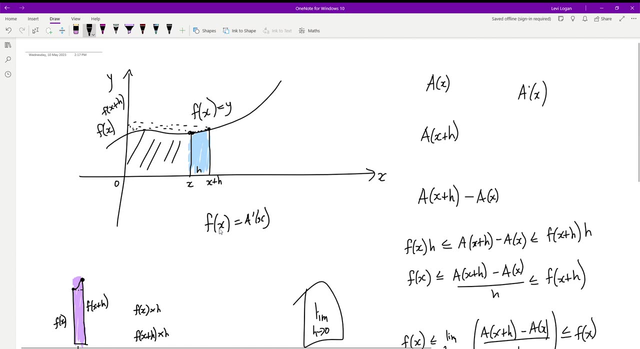 to f of x, then f of x is equal to a dash of x. So let's take this up here. and what does this actually mean? So our function, this function here, is the derivative of our area function. So if we want to undo a derivative, we have to integrate, don't we? So therefore,